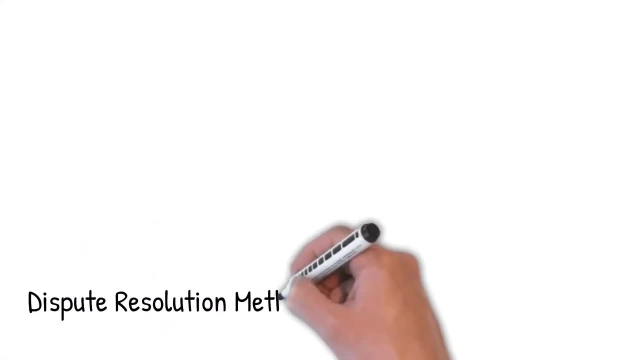 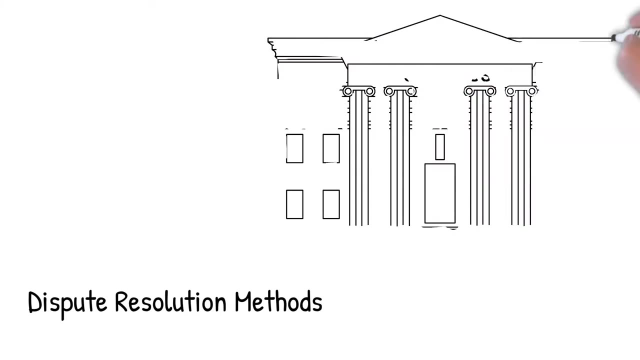 Welcome to our video on dispute resolution methods. To be frank, we hope that you'll never be in a position where you need to engage with dispute resolution on any of your construction projects, But we do believe there's no harm in understanding the different options available to. 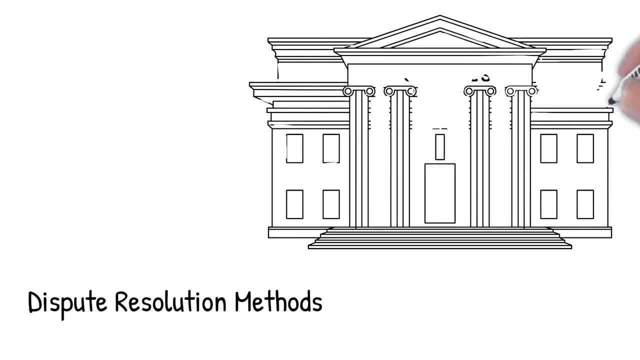 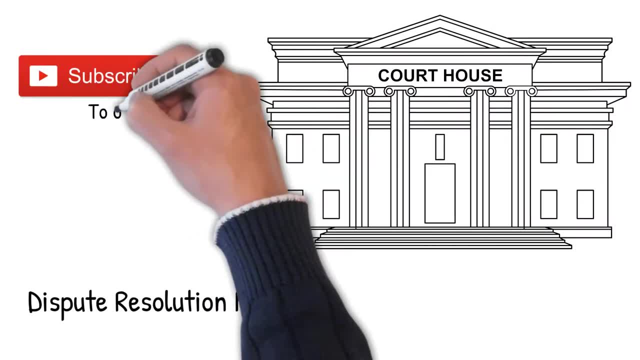 you and your company if the worst should happen, and there's no way to come to an agreement without it. You may notice that some of the other videos on our channel include tips and techniques on how to try and avoid dispute resolution, namely: site records, disallowed cost and risk management. 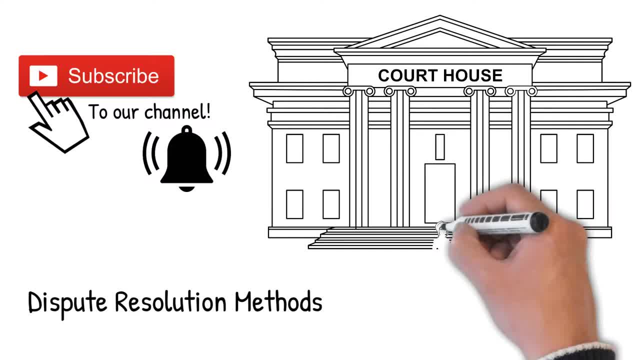 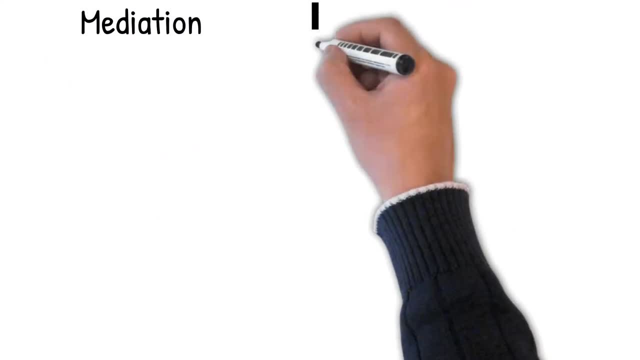 But if you've exhausted all of these options, this may be the video that you now need. The good news is that there are a number of alternative dispute resolution methods open to contractors and subcontractors over the traditional, pricey litigation route. Firstly, mediation: Mediation is a very common method of dispute resolution within the construction. 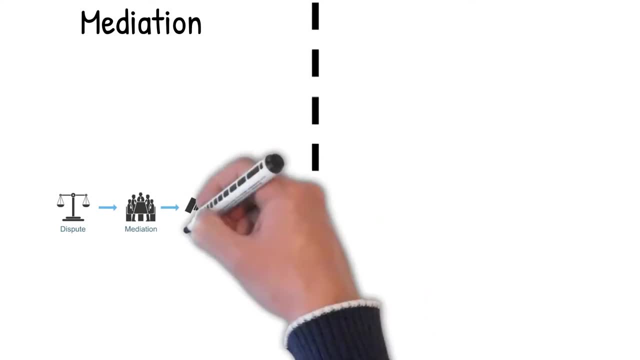 industry and is often the first method parties will attempt. It consists of an independent person who will facilitate a discussion between two parties in the hope they can come to an amicable agreement. It is important to note that the mediator will not pass judgment or make a decision. 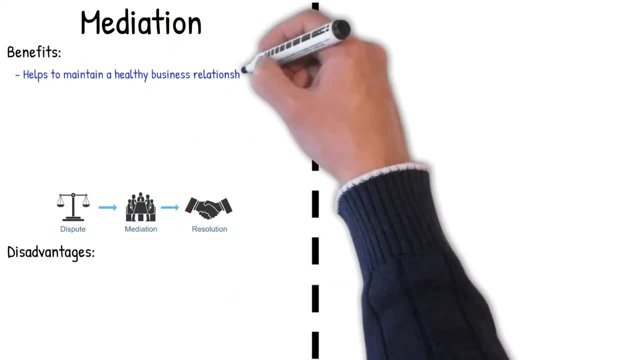 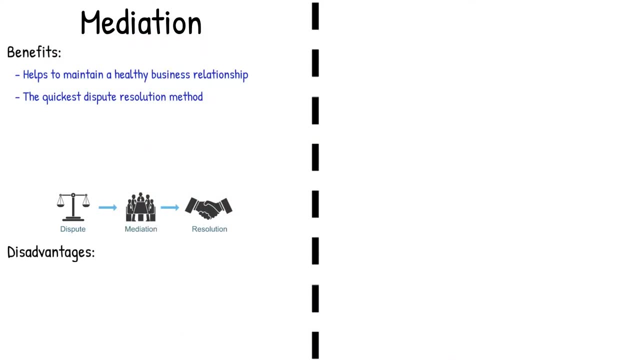 Benefits A useful method in helping to maintain a healthy business relationship. Once mediation is confirmed, it's generally very quick to reach an agreement. Most mediations only last one or two days. Everything that has happened and that is said in mediation is completely confidential. Costs considerably less than litigation. 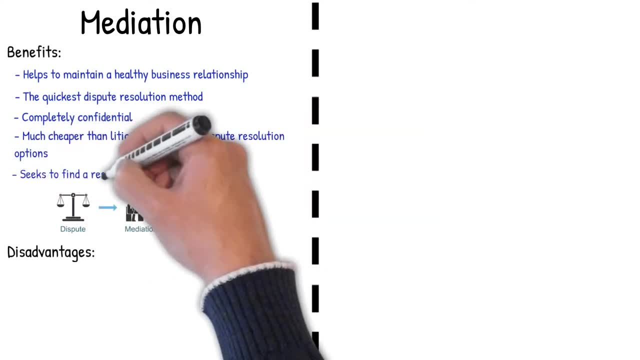 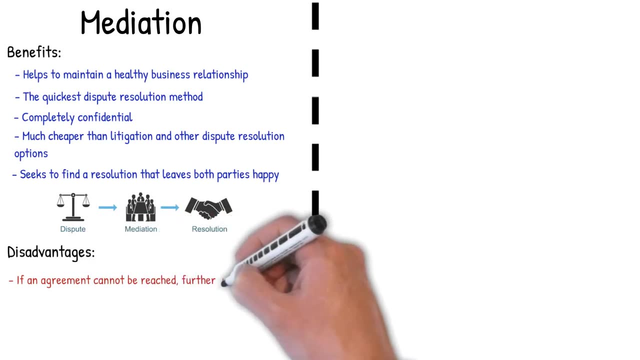 And finally, the mediator always encourages a solution that suits both parties and hopefully allows them both to walk away happy Disadvantages. If the parties cannot come to an agreement, further action will be required and the cost of the mediation will have been wasted. When an agreement is not possible, 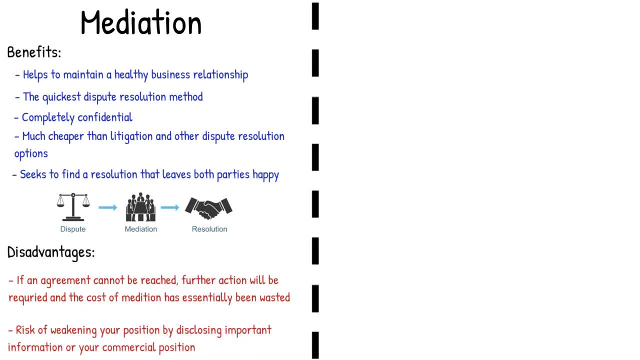 parties are worried that they may have disclosed sensitive and important aspects of their argument or commercial position, which weakens their position when conducting further dispute resolution methods, or if it goes all the way to trial Adjudication. This option means a neutral third party will give a decision on a dispute. 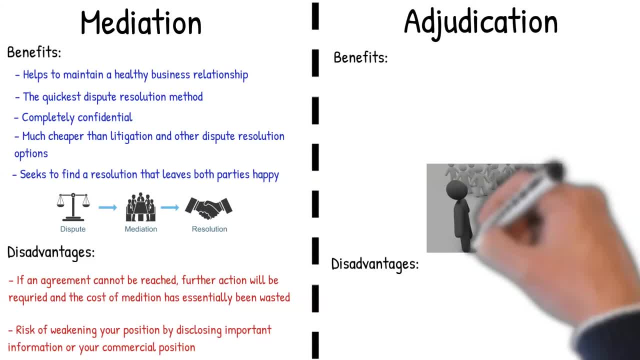 The decision made by the adjudicator will be binding unless the losing party decide to take the case further and engage the arbitration or litigation process. Both parties are allowed to refer a dispute to an adjudicator under the Construction Act 1996.. Benefits: 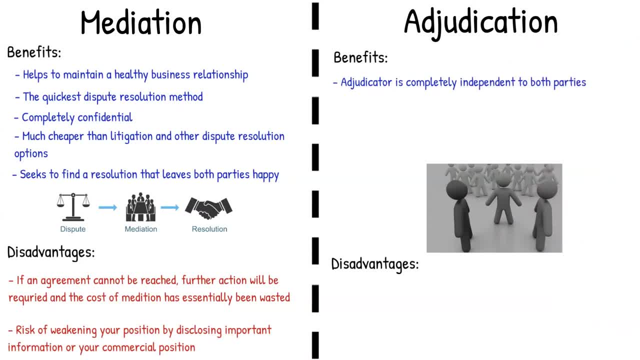 The adjudicator is completely independent to both the disputing parties. Adjudication effectively acts as a pay-now-argue-later mechanism, which helps maintain the company's cash flow throughout the dispute And, finally, it's inexpensive compared to court proceedings. 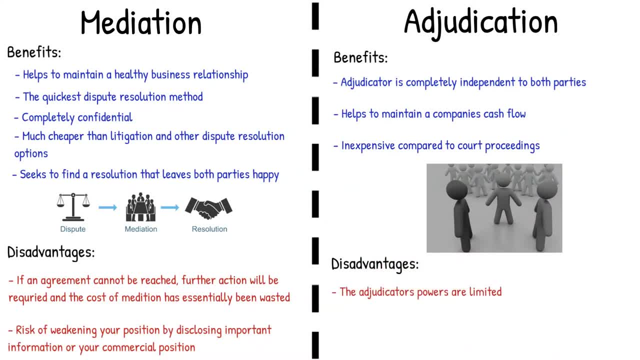 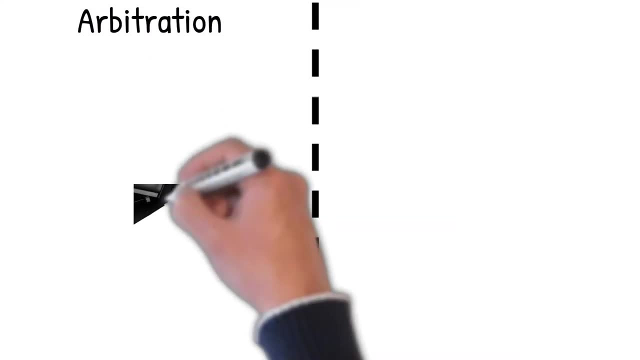 Disadvantages. The adjudicator's powers are limited, which may result in further dispute resolution methods being necessary. Court proceedings will be required if the losing party fails to pay or adhere to the outcome reached. Arbitration- Arbitration is again where the party agree to refer the dispute to a third party. 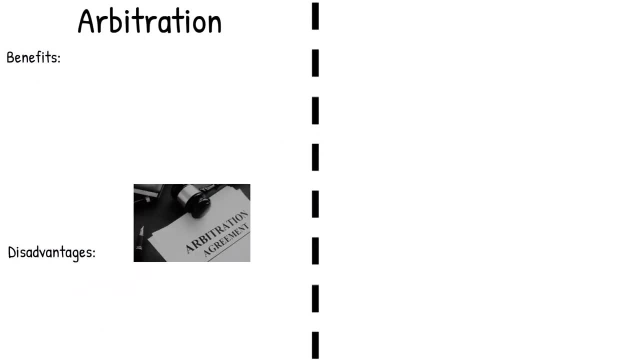 but here the disputes are judged and analysed on the basis of facts, available documents and relative principles of the law governed by the Arbitration Act 1996.. Benefits: Arbitrators hold stronger powers than adjudicators. Arbitration is a completely confidential process. Both parties have a say on who the expert arbitrator. 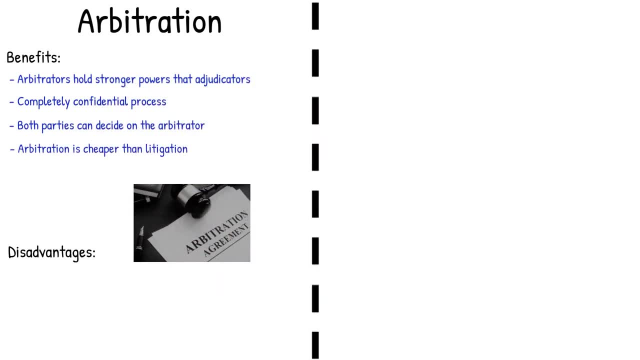 is Compared to court and full-blown litigation, arbitration is a cheaper option And, finally, more flexible than court proceedings. Disadvantages: There are limited appeal rights. when using this method, Parties must bear the cost of both the arbitrator and the venue. 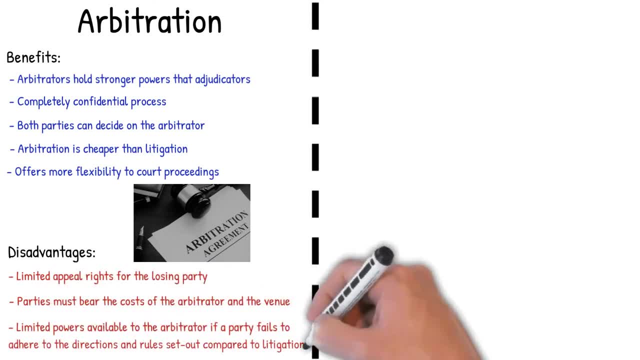 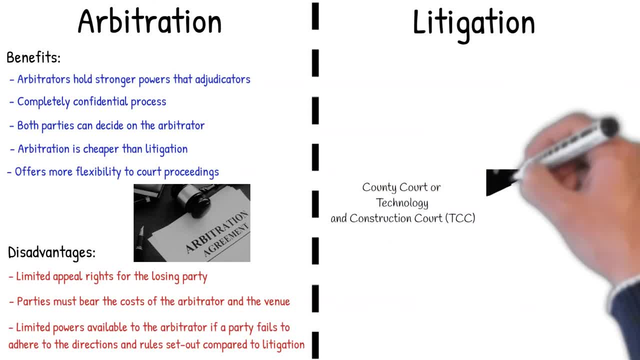 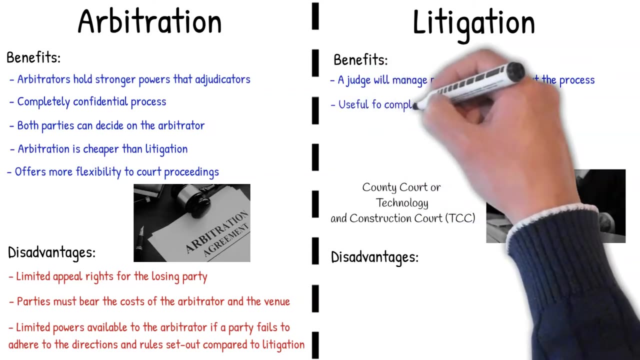 The dispute gets referred to either the county court or the technology and construction court. If the dispute is under £250,000, then the court used will always be a county court Advantages Throughout the process. the judge will manage proceedings, Useful for complex issues and disputes where a great deal of money is at stake. 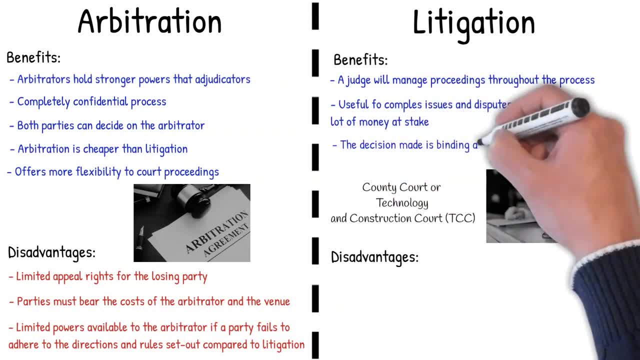 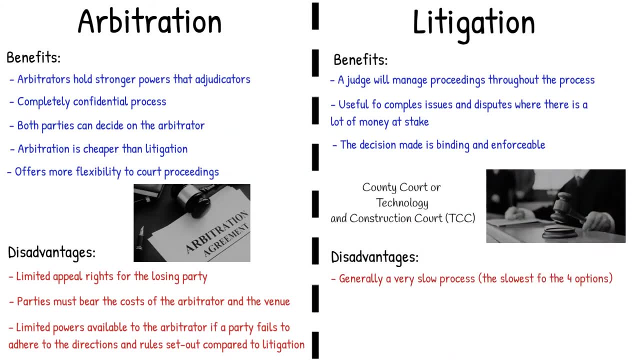 Finally, the parties will obtain an enforceable and binding decision. Disadvantages: It is generally a very slow process. It is extremely often the most expensive way to resolve any given dispute. Unlike the arbitration and adjudication methods, the proceedings are generally public. 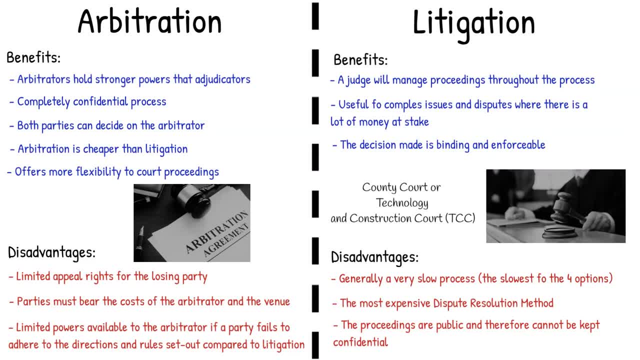 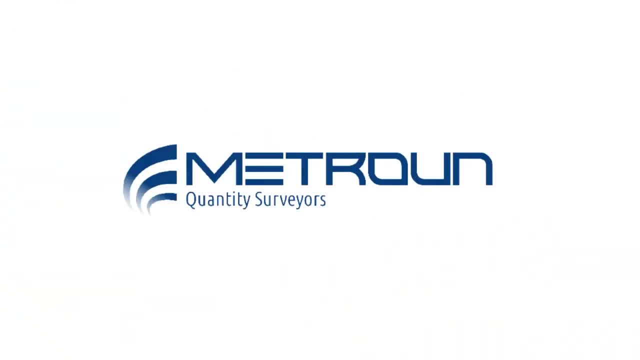 and therefore cannot be kept confidential. Click on the links in our description below to view videos on how to avoid having to use any of these methods. Matrone a commercial hub to your business.